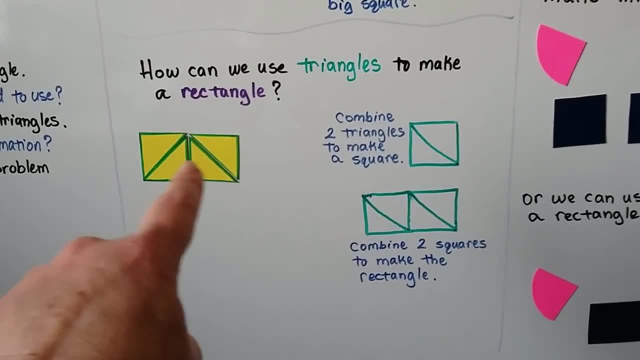 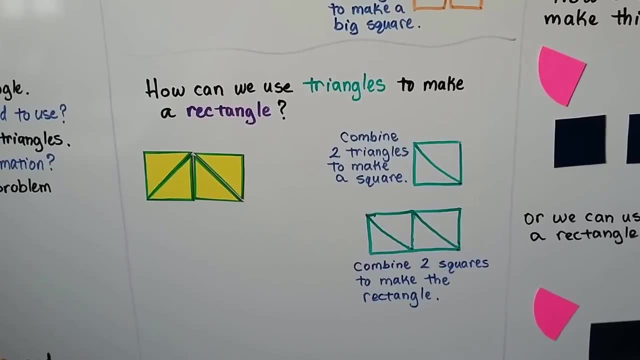 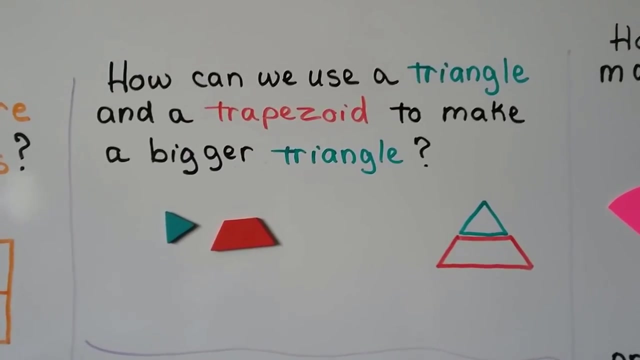 Okay, Look at how these two triangles made a bigger triangle, didn't they? These two in the middle? But if we put all four triangles together, we can make a rectangle. How can we use a triangle and a trapezoid to make a bigger triangle? All we have. 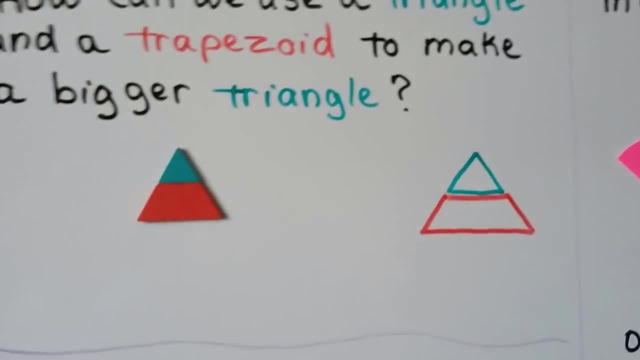 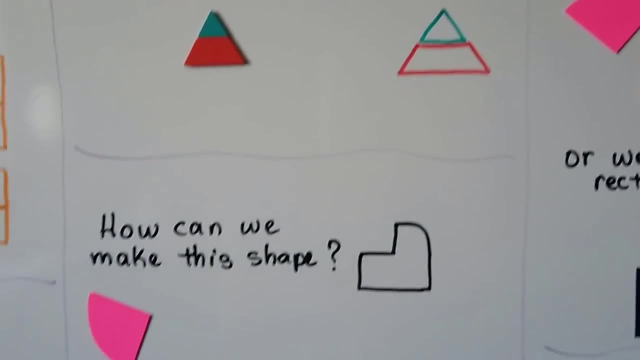 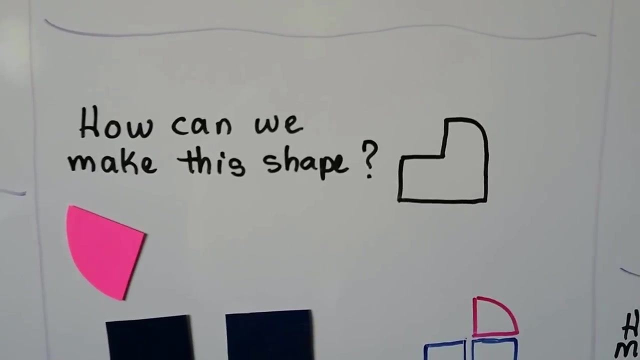 to do is put the triangle on top of the trapezoid. Look at that And it makes a bigger triangle. OK, How can we make this shape? I thought this looked like a baby bassinet, Doesn't it? Can you see the shapes that are in this shape? 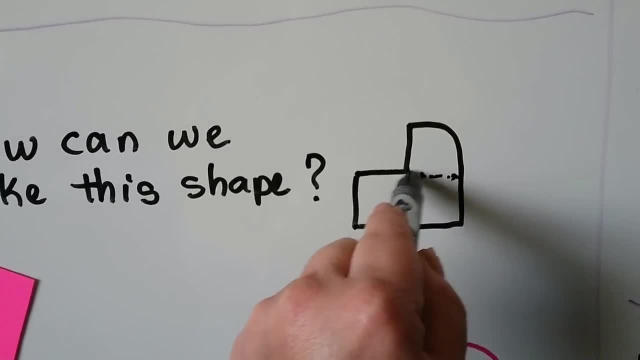 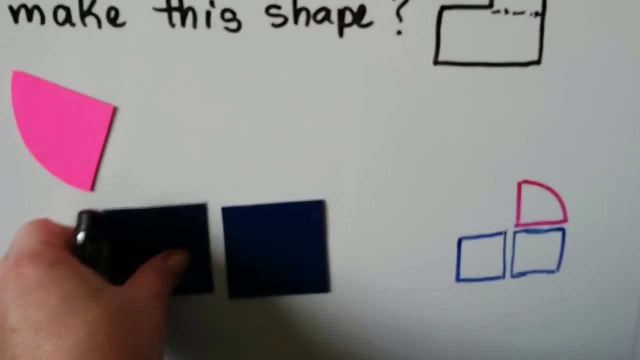 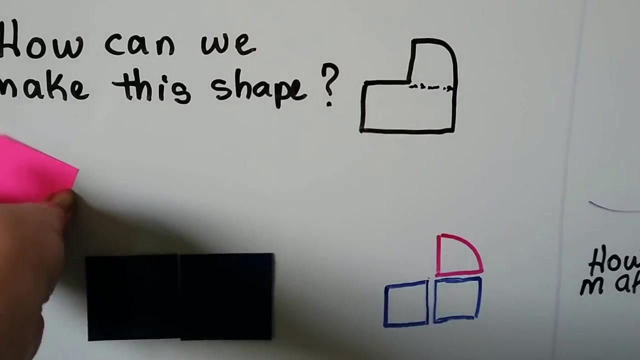 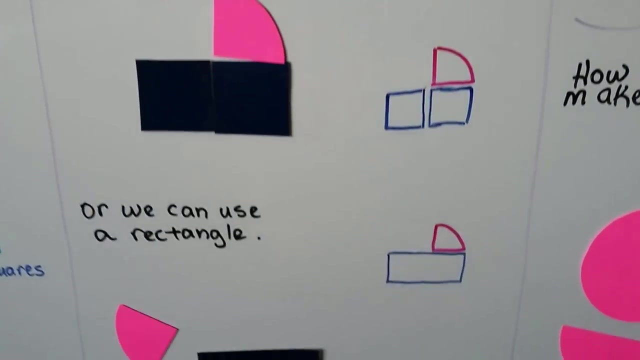 What if we drew a line along here? Do you see the rectangle? We could make the rectangle with two squares and we can use part of a circle to finish it, Or we could just use a rectangle. We could use a rectangle and just put this: 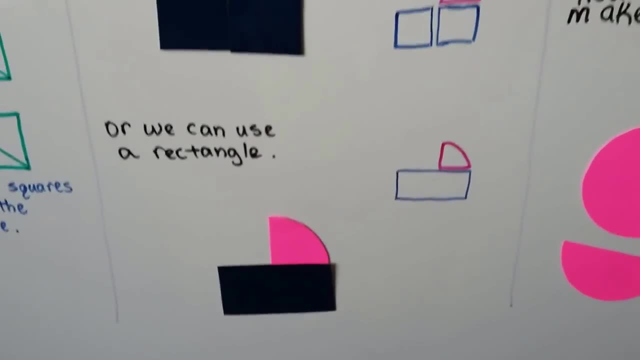 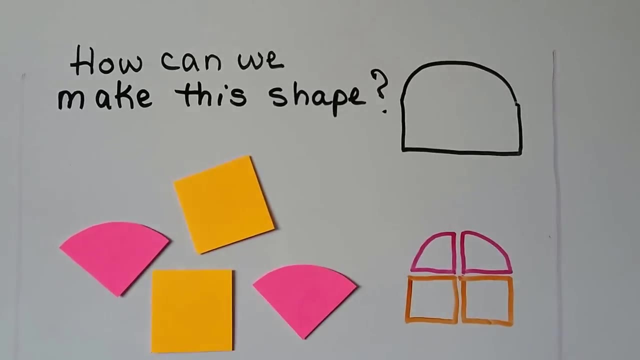 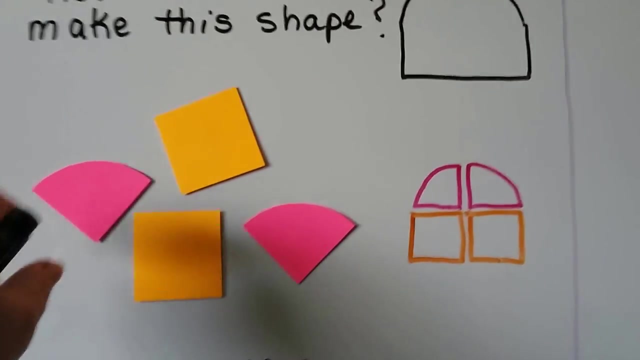 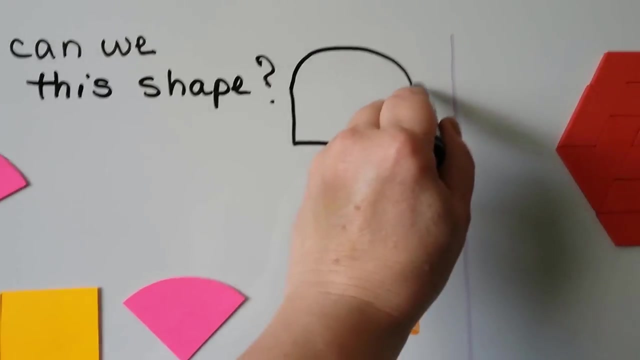 right here, couldn't we? That would make that shape. How can we make this shape right here? Well, it's got the corners down here, so we know the squares can go on the bottom to make a rectangle and the top part looks like a semicircle, doesn't it? 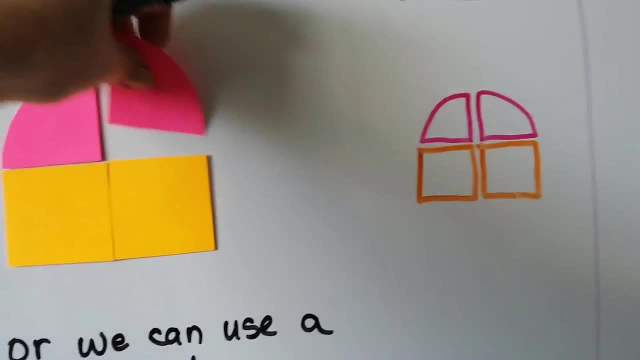 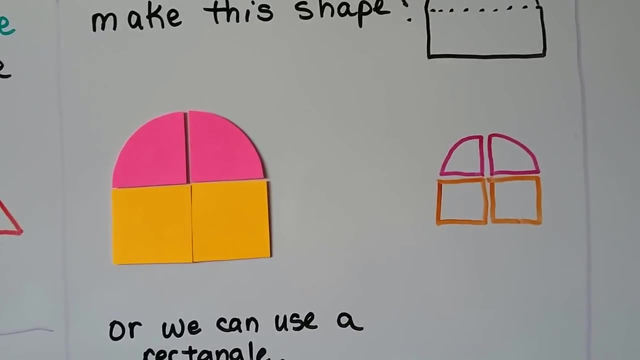 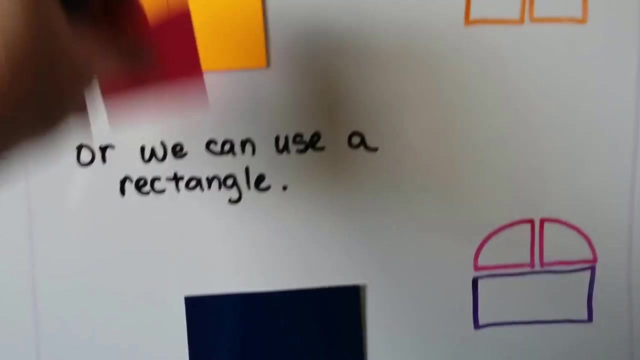 We can make a semicircle with the parts of a circle. It almost looks like windows of a house. We could also use a rectangle. We could just use the rectangle for the bottom part and the two parts of a circle to make a semicircle. 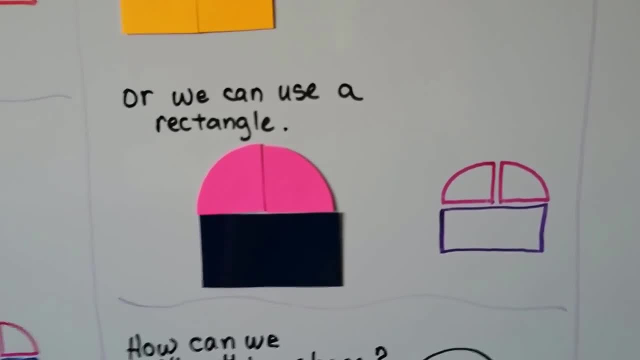 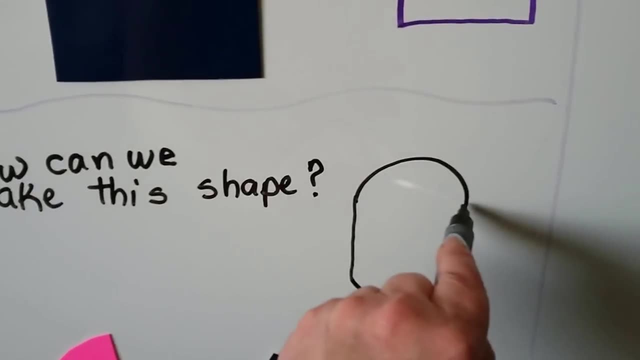 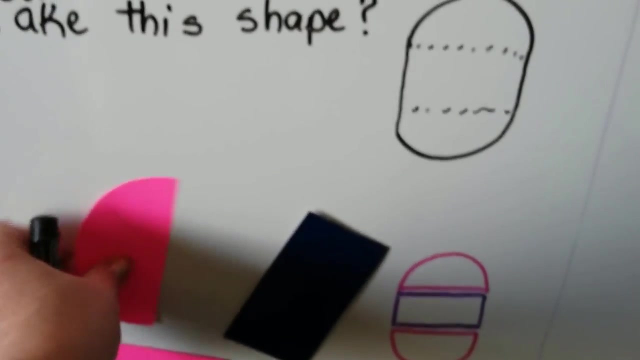 and we could make the same shape. How can we make this shape? What if we drew lines going across like this and like this? Do you see the shapes? We have a semicircle on top, Then we have a rectangle, Then we have a semicircle on the bottom. 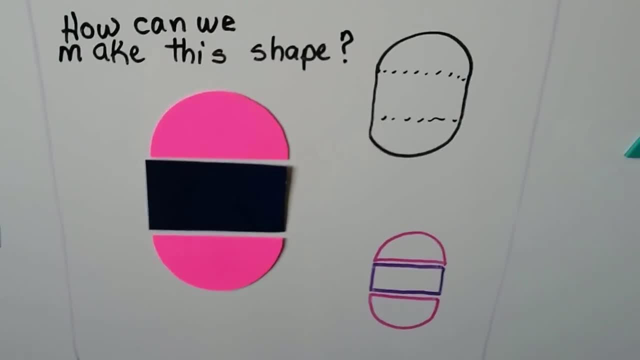 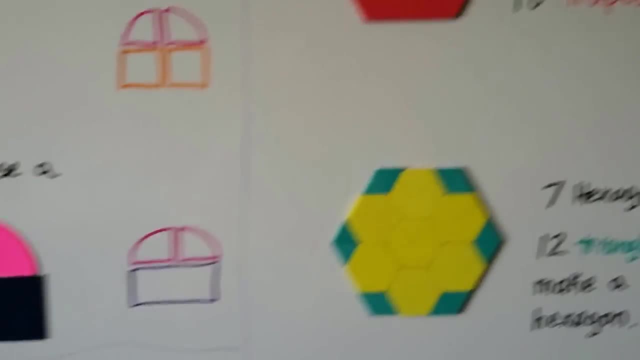 Then we have a rectangle, Then we have a semicircle on the bottom. It looks like a rectangle sandwich, Or like a hamburger, doesn't it? Now, I had fun making this. I made a big hexagon by combining 18 trapezoids. 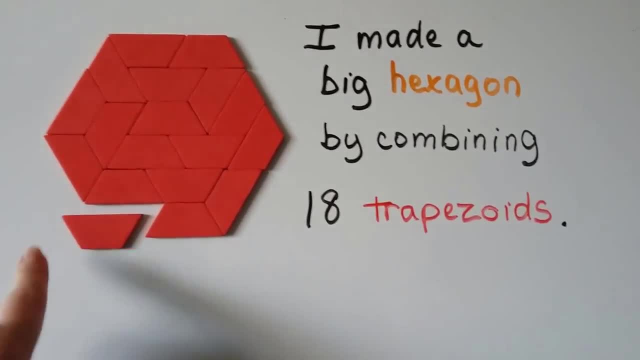 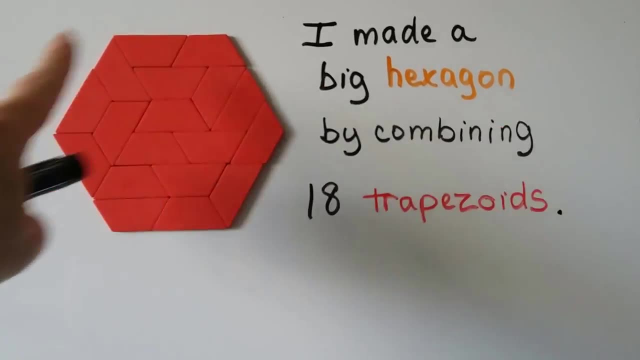 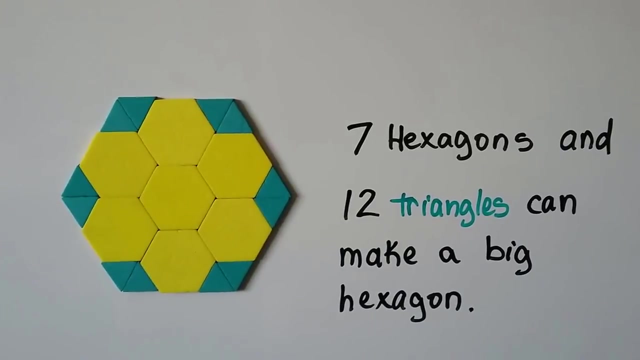 I was happy that I had enough red trapezoids to do this. I was afraid I was going to run out. I just put them together and it made a very big hexagon. Then I took 7 hexagons and 12 triangles and made a big hexagon. 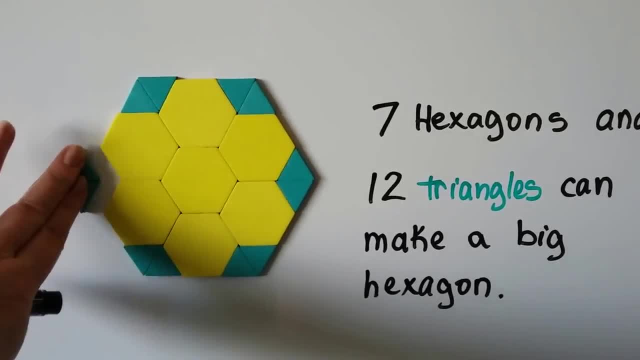 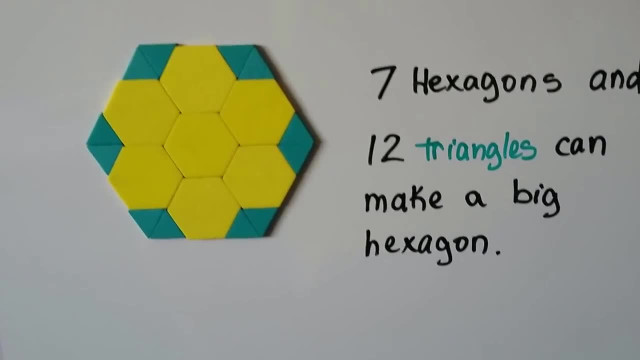 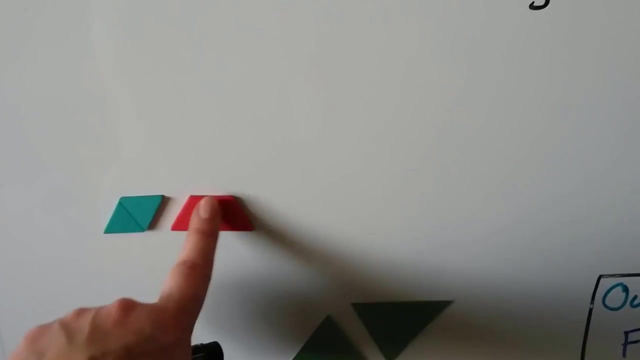 This looks like a flower, doesn't it? I put the triangles together. See, I had a trapezoid and I put 2 triangles together to make a rhombus, And when I put them together I made a wider trapezoid. 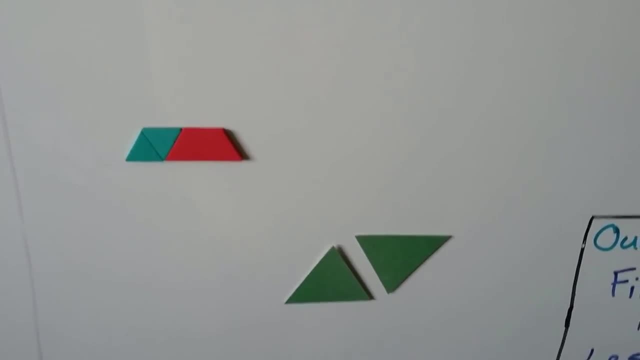 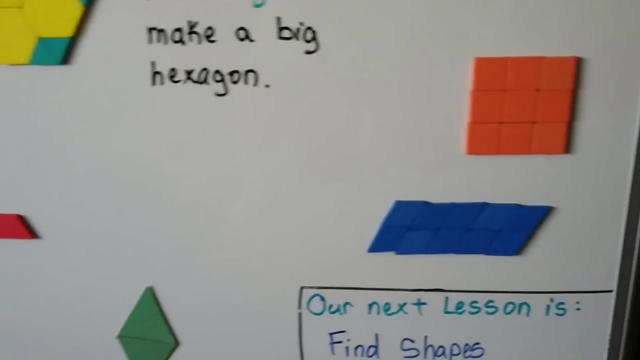 See that I can take 2 triangles and put them together and make a rhombus. When I turn it sideways, it looks like a diamond, doesn't it? Doesn't it look like a diamond shape? So we can make new 2-dimensional shapes from other shapes. 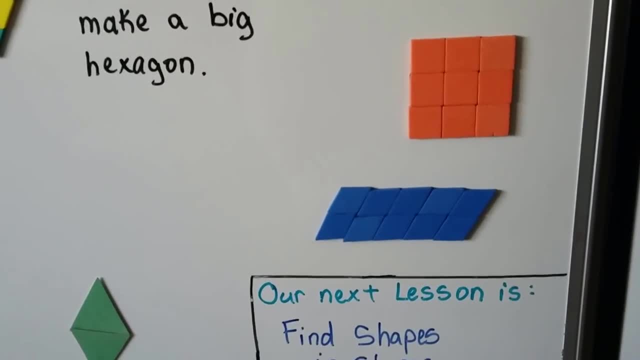 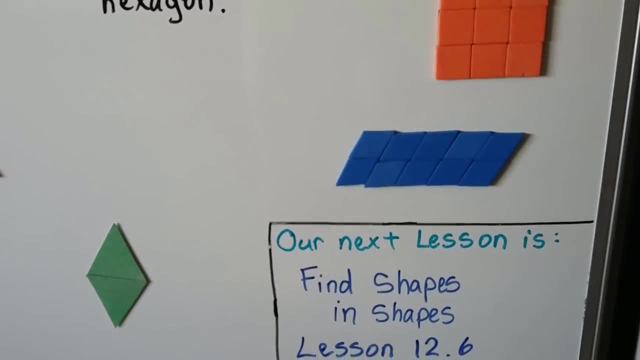 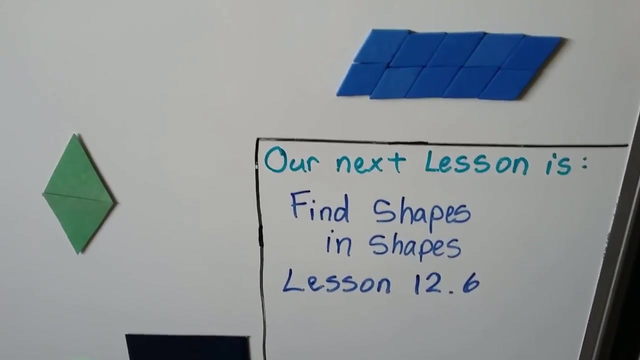 Here's 9 squares that made a big square. Here's a lot of rhombuses that I put together to make a very long parallelogram. Our next lesson is find shapes in shapes. That's lesson 12.6.. So, just like we did here, where we found that there was a semicircle up here, 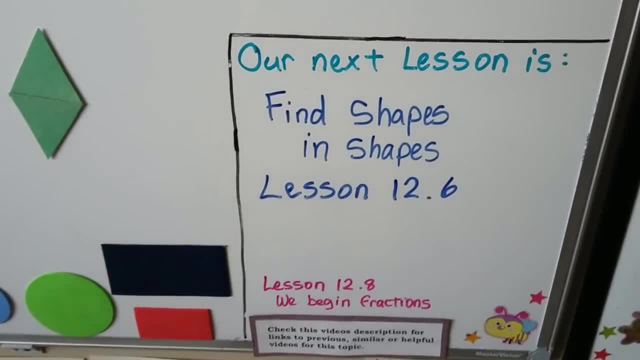 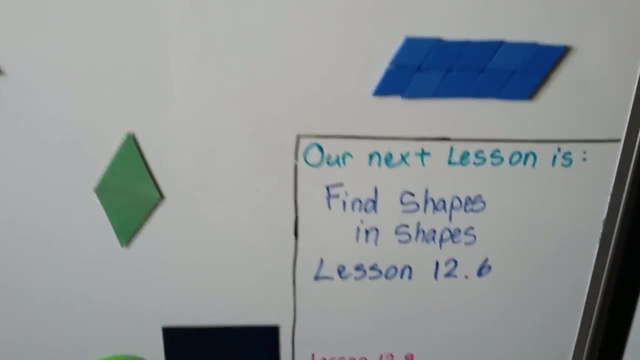 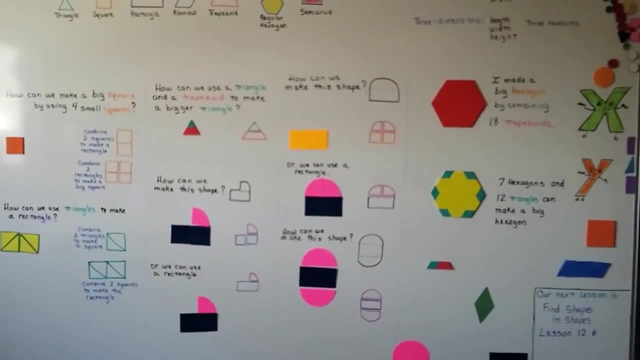 that's what we're going to be doing in the next lesson. Okay, And this is all leading us towards 12.8, where we're going to begin learning about fractions. That's coming soon, So you can make your own shapes, and you could buy some shapes from the Internet. 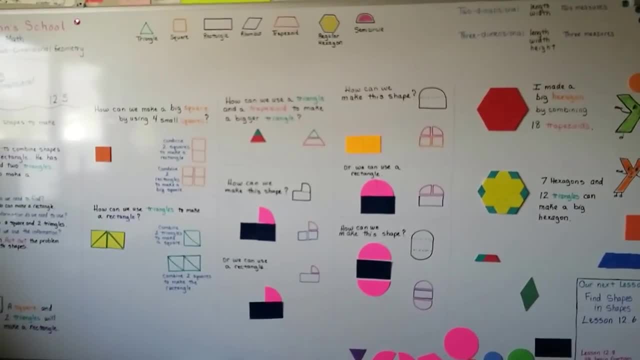 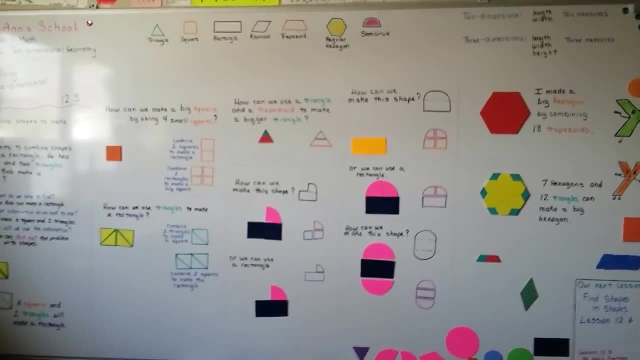 I use the Learning Resources brand. You can get them on Amazon or on the Internet, or you can even buy them from Learning Resources, And you can get them magnetic or not magnetic. And you can get some poster board and make your own, like I said, or construction paper. 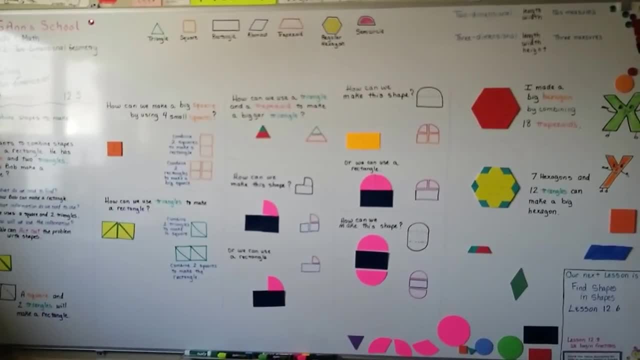 Okay, So have a great day and I'll see you next time. Bye.